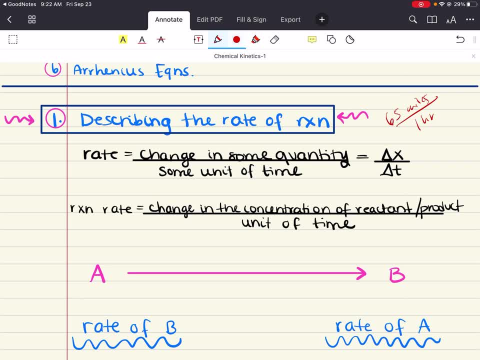 notice that you have some unit of time in the denominator to describe the rate at which you are driving. It's the same thing now when we try to apply this to a chemical reaction In a similar way. actually, the rate of a chemical reaction can be described as the change in the concentration. 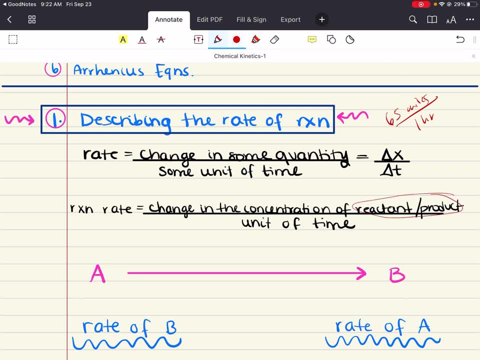 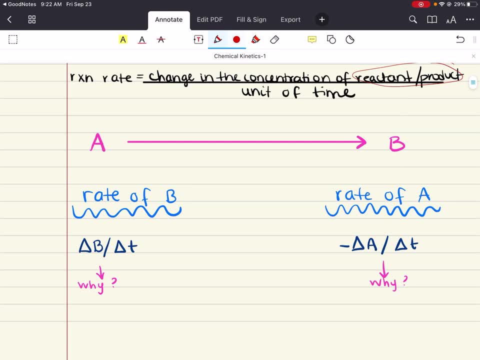 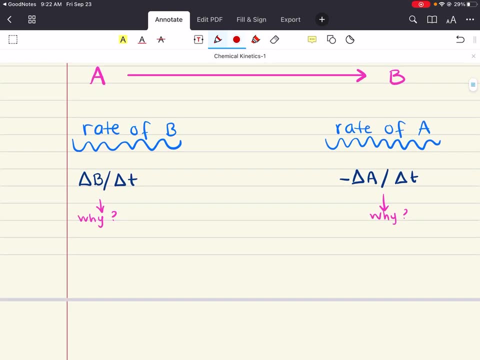 of a reactant or product over some unit of time. So if we take this reaction right here, reactant A going to product B, we can describe the rate of this reaction first. We can do it by in terms of changes in the concentration of the product B over some period of time. 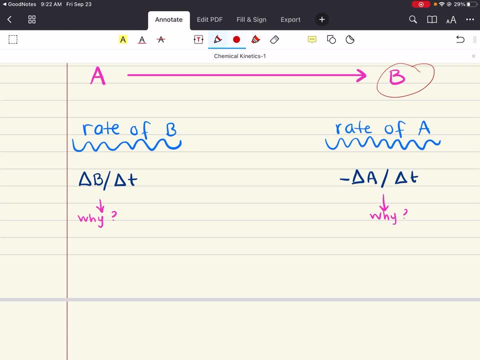 If we're going to describe the change in concentration over some period of time for product B, what we're going to rate is change in concentration of product B over some time, And we have a positive sign here, by the way, just letting you know. I'm going to explain that. 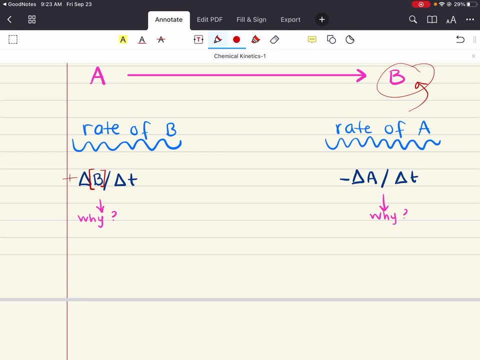 in a second. If we were to describe the rate of this reaction in terms of the change in concentration of our reactant A, it's going to be slightly different. It's going to be minus change in concentration of A over a specific amount of time, And this expression describes. 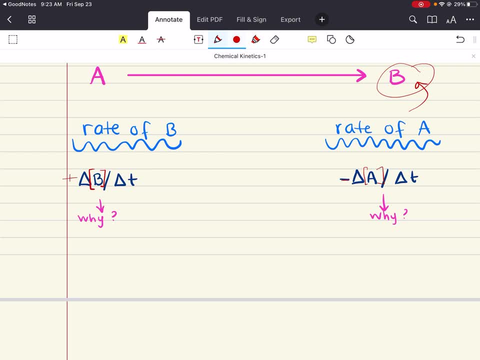 the rate at which the reactant is being consumed. Because the whole point of this reaction is you're starting with A and the reactants are being converted to products. So why is there a negative sign here and a positive sign here? Well, we can just fall back to our idea of what change is defined as Change in some quantity is. 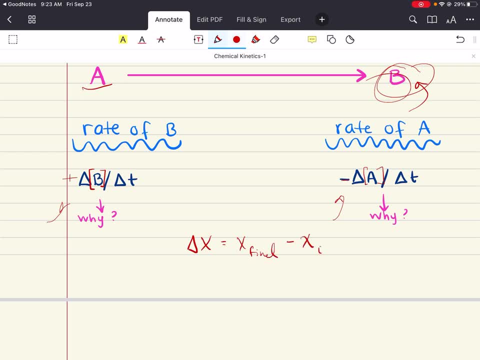 that quantity final minus quantity initial, All right. So this is going to be negative because the reactant A is going to be consumed to form product B, All right. So you're kind of like losing reactant as the reaction proceeds, which is why there's a negative when we describe the rate. 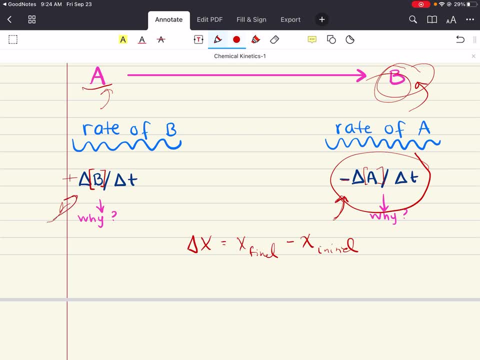 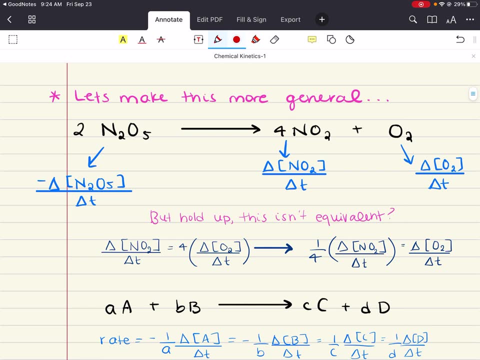 of a reactant, Why there's a positive sign when we do that for the product. All right, Now we can look at this in a more general scenario, like a more specific one. actually, We can look at this reaction right here. We're studying the following: All right, We have this reactant that forms two products. 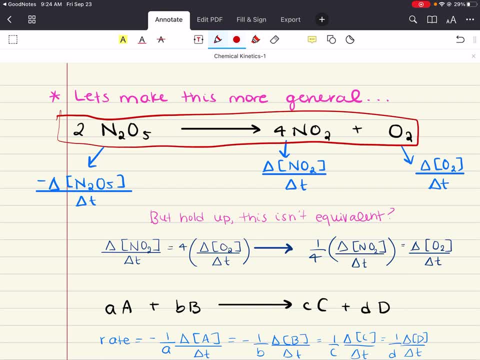 The reaction rate can actually be described in terms of any of the reactants or products here. For example, we can describe the rate in terms of how fast N2O5 is being consumed, All right. In terms of how fast NO2 or O2 are being formed, All right. And we could actually write this for. 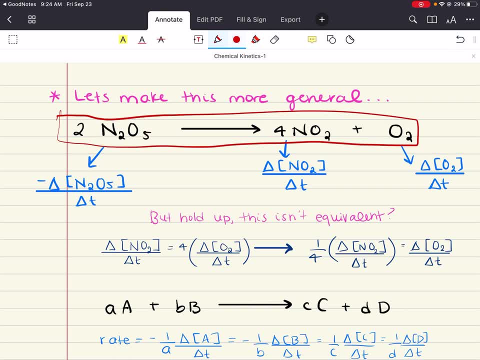 each one of these terms. So for the reactant N2O5, we can write the following rate: The rate is equal to minus the change in the reactant's concentration over time. We can do this for the product NO2.. All right, Plus- there's a plus there- Change in concentration of NO2 over time. Same thing for O2.. 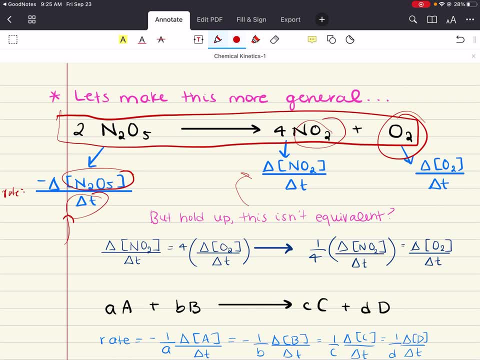 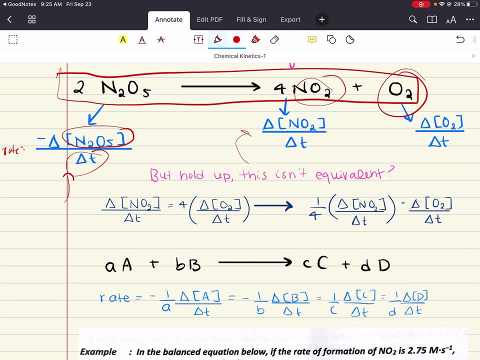 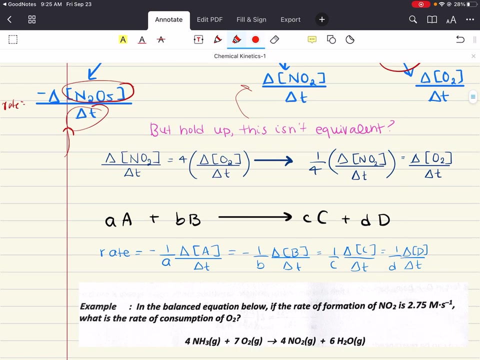 Change in concentration of O2 over time. Now, one thing that's really important to notice here is that these terms are not equivalent. The balanced equation here indicates that, hey, four moles of NO2 are formed for every one mole of O2 that is formed. So then we want to write some form of equivalence here. All right, What? 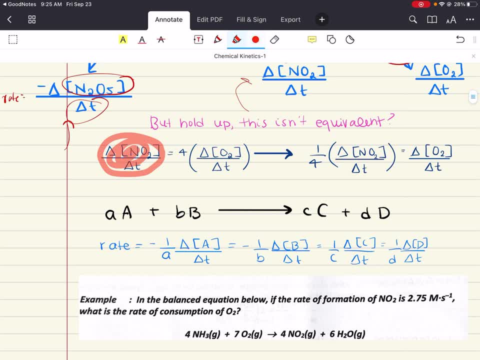 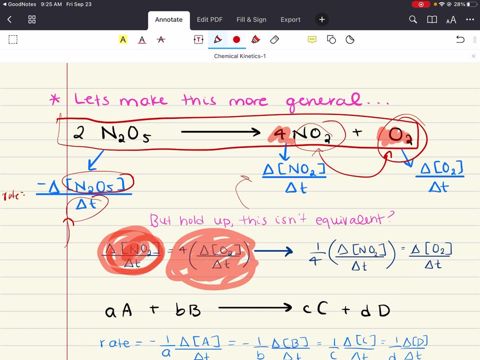 we can write is that for the rate of NO2, for every NO2 that we might create or produce. All right, We're trying to write an equivalence kind of expression here. All right, So that means if there are four NO2s that are being formed, all right. for every one O2, that means that NO2 is. 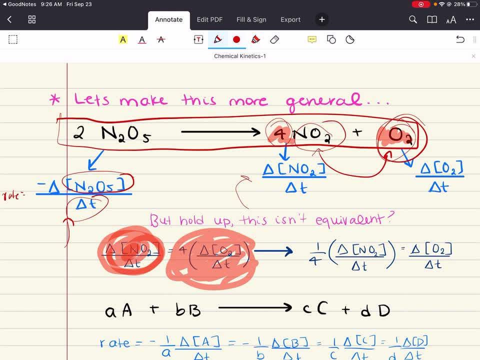 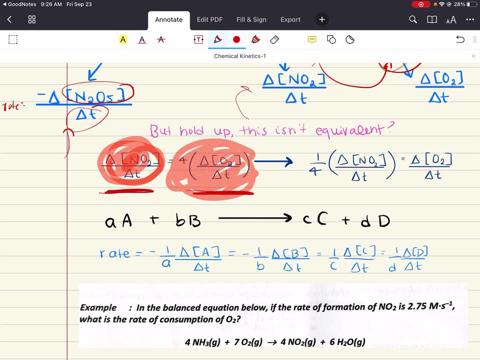 being formed four times faster than O2.. So if we're trying to write an equivalence of rate for NO2 and the rate for O2, NO2 is being formed four times faster than O2.. So if we're trying to write an equivalence for O2, to make this equivalent we're going to add a four, all right, as a. 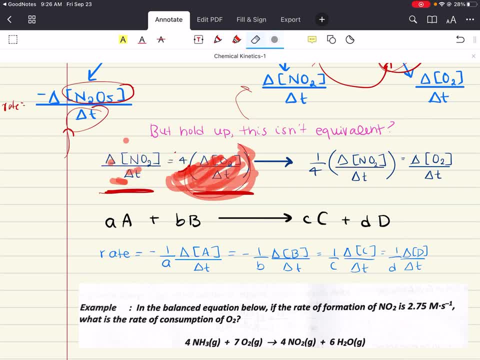 coefficient to the O2.. So now they're actually balanced. All right, So we have the following expression now, where there's a four associated with the change in concentration of O2 to make it equivalent to this. All right, Now what we can do is actually then divide both sides by four. 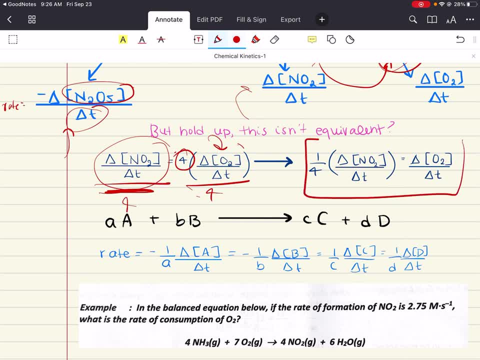 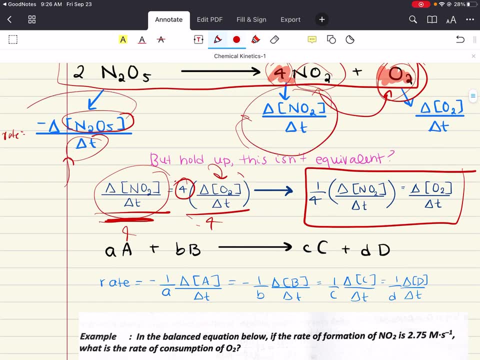 so that we can move the four to the other side and we can get the following expression: Now we can do this for any one of these. actually, We can relate this product to this reactants, and so on and so forth, And we have different coefficients that we have to account for. All right, Now these examples. 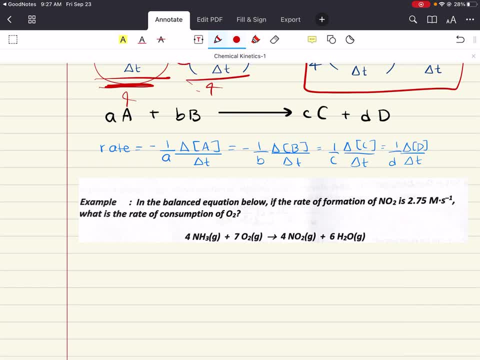 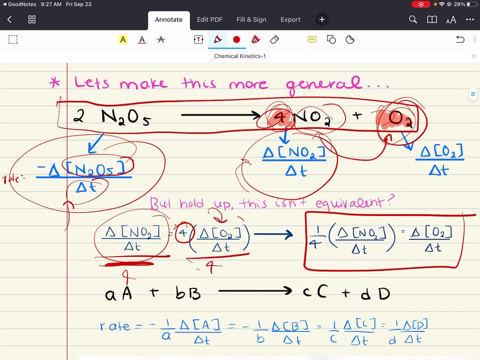 ultimately show how the coefficients in a balanced equation are going to become reciprocal when the reaction rate is expressed in terms of various reactants or products. which means if we're trying to relate this to this, all right if we're trying to write an expression. 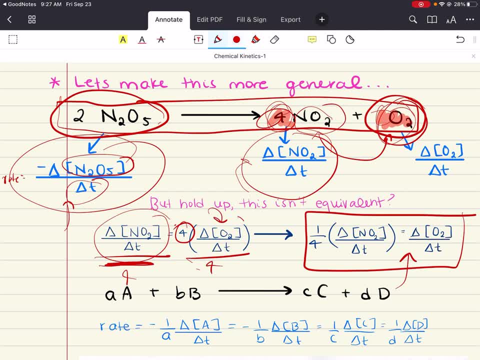 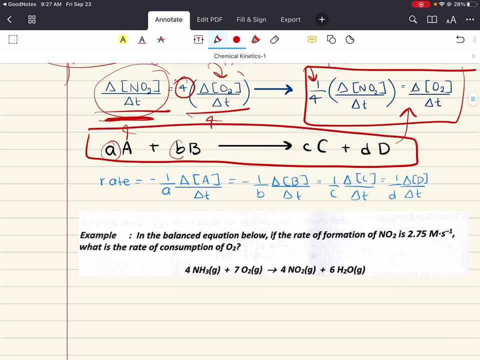 similar to the one we wrote for the two products, but for one reactant and one product. just know that these coefficients turn into reciprocals when they're associated with their molecule. So if we have a reaction that looks like this, where all the lowercase letters are: 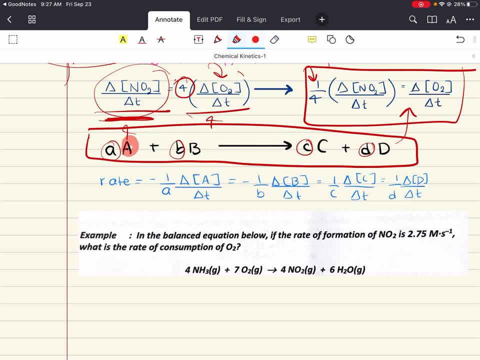 coefficients associated with the molecules which are in big letters. All right, And we want to write a reaction rate for every single one of these reactants and every single one of these products. We can do this with the information that we have just learned. We can write that the rate for reactant molecule A 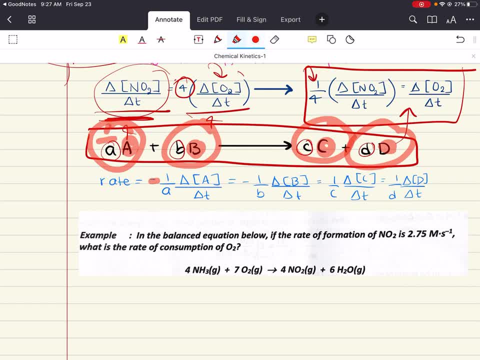 all right, we have to have a negative for reactants. is one over A the reciprocal of that change in concentration of A over time? We can do it for this one as well. right here that I'm going to actually highlight in yellow: All right. Reciprocal of that coefficient: one over B minus. 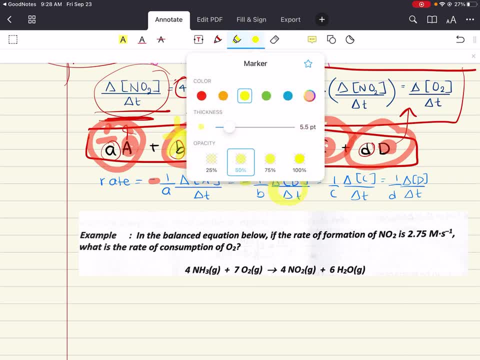 because it's a reactant, and then change over concentration of B over time. Same thing with the products one over C, which is the coefficient change in the concentration of molecule C over time. Same thing with this one. one over D- change in. 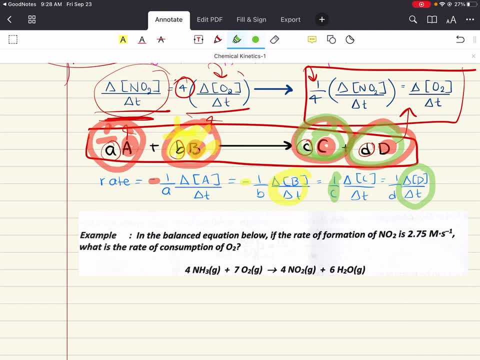 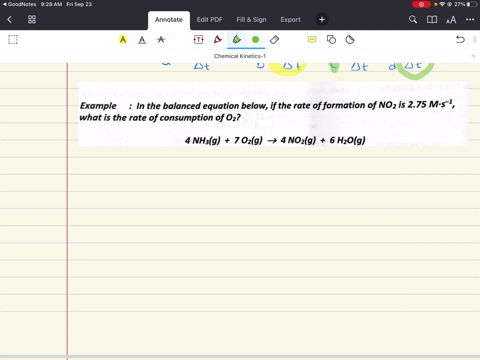 concentration of D over time. And so now we have a quick way of expressing a general equation for the reaction rate for this reaction. All right, Fantastic. Let's put this into action. now. Let's actually do a real practice problem. This problem says in the balanced equation below: if the rate 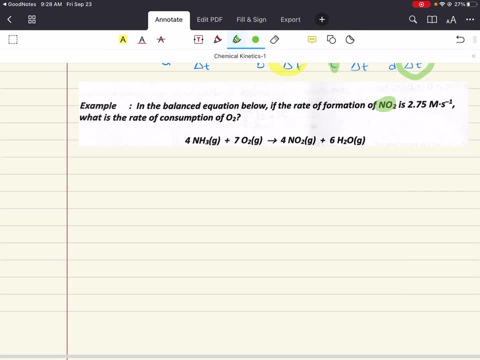 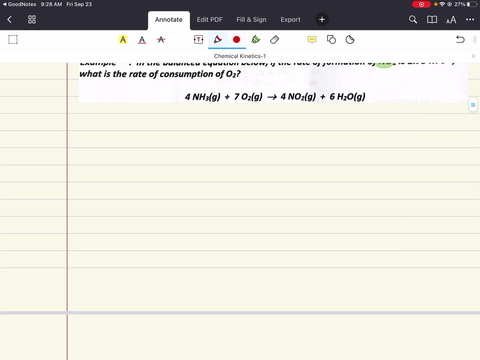 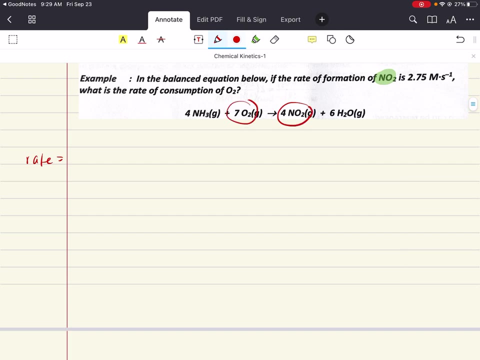 of NO2 is 2.75 molar per seconds. what is the rate of consumption of O2?? All right, For practice sake, let's write the whole rate for this whole reaction, even though we're only paying attention to NO2 and O2.. We're just going to write the whole thing out. All right To write it. we start off. 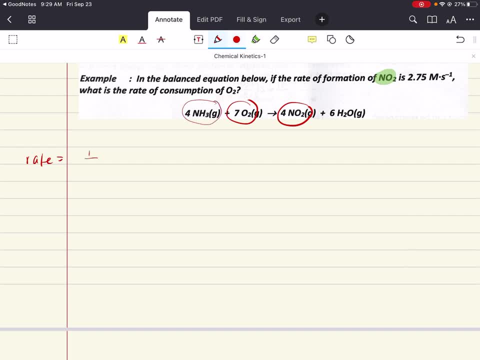 with this reactant. All right, That four is going to be the reciprocal of that for this reaction rate. It's a reactant, So minus change in concentration of ammonia Over change in time. Do this for O2 as well. Reciprocal of the coefficient minus because it's. 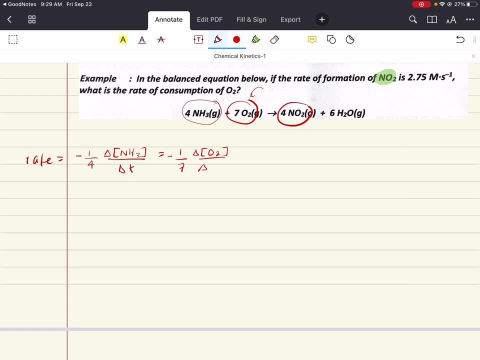 a reactant, Change in concentration of O2 over time. All right, Now we're getting into the products. It's going to be pluses, but reciprocal of that coefficient. So one over four Change in concentration of NO2 over time. And then similarly for that last one, water, One over six: Change in 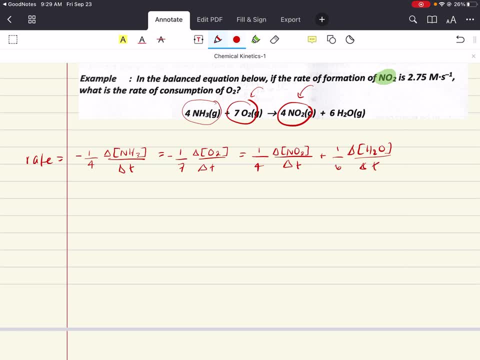 concentration of NO2 over time. Fantastic. Now again, our problem is really focusing on just two of these NO2.. All right, The rate of formation which we are given, And then we're trying to find the rate of consumption of O2.. So really the only part of this reaction rate that we're focusing on. 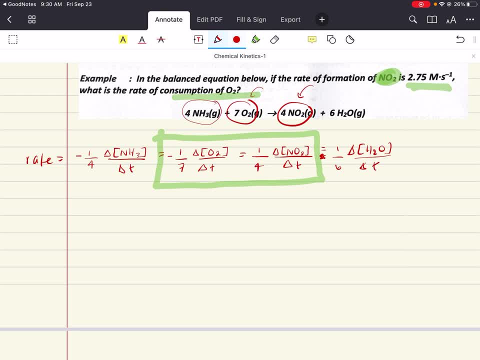 here is this, And this is not supposed to be a plus sign. This is an equal sign. I'm so sorry. All right, This is the only part of this reaction rate that we're going to be dealing with. All right, So we have minus one over seven. Change in concentration. 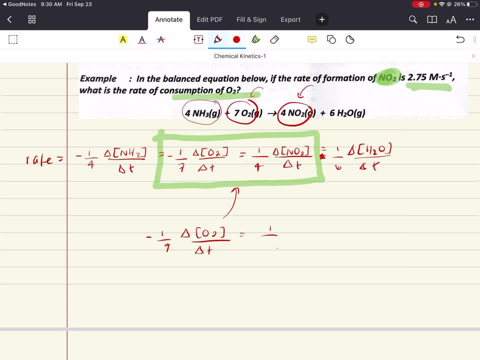 Of O2 over change in time is equal to one over four Change in concentration of NO2 over time. We want to find the rate of consumption of O2., Just O2.. All right, So to do this, we're going to actually move this minus seven over to the other side. We're going to multiply. 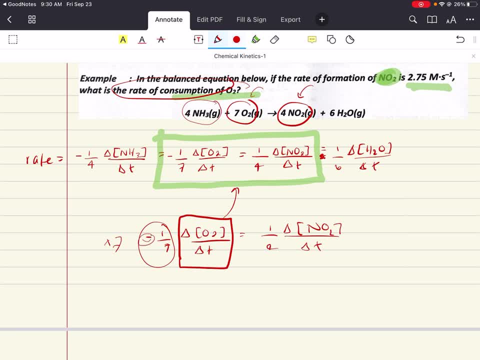 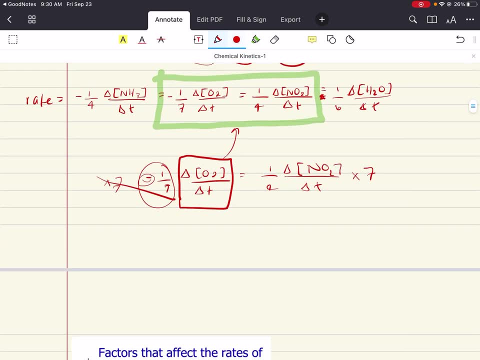 each side by seven. Actually, we're going to keep the negative here. It doesn't matter, All right. So we're just going to get rid of the seven. We'll multiply this side by seven. We'll multiply this side by seven. All right, Because what you do to one side. 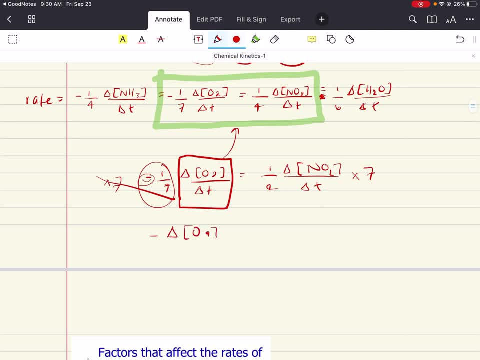 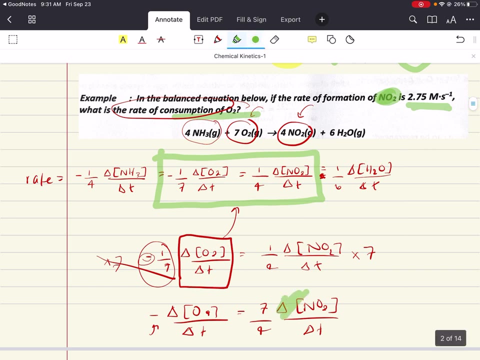 you do to the other. Now we get that the change in concentration of O2 as it's being consumed- which is what that negative means- is going to equal seven over four change in concentration of NO2 over time. Hold up a second. We know what the rate of formation for NO2 is. We know what this. 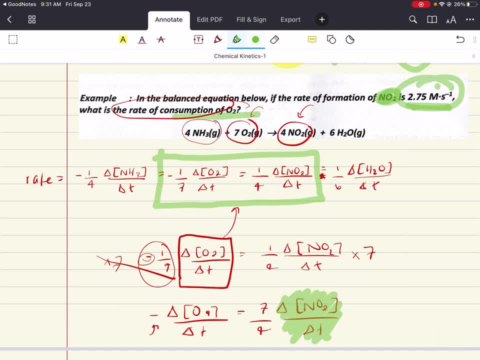 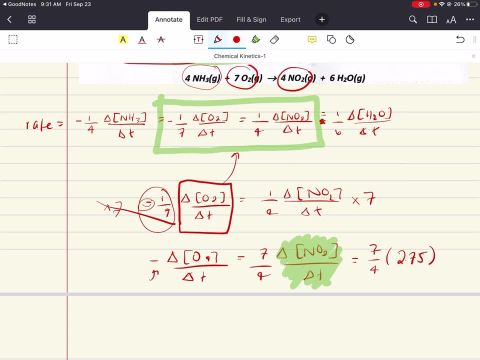 whole term is. It is simply 2.75.. So what we can do now is plug that in and we get seven over four times 2.75.. Plug that into a calculator. You're going to get the rate of formation of NO2 over. 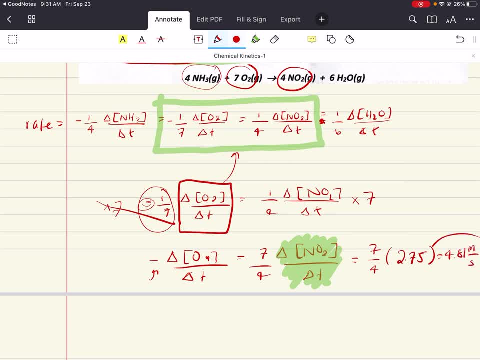 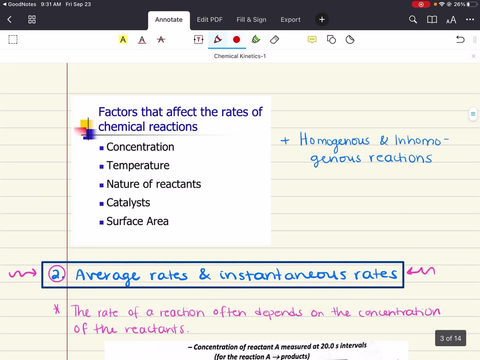 4.81 molar per second. This is the rate of consumption for O2.. And that's it. We have solved the problem, Fantastic. Now there are also things that are going to affect chemical reactions. There's factors that are going to influence the rate of a chemical reactions. 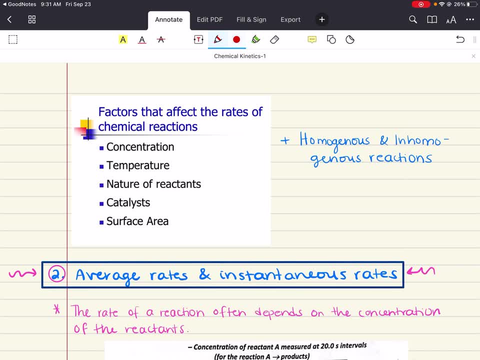 And there are several factors. One of the most important one is temperature In general. the higher the temperature, the faster the chemical reaction. All right, So keep that in mind. That's really important That temperature is one of the larger factors. 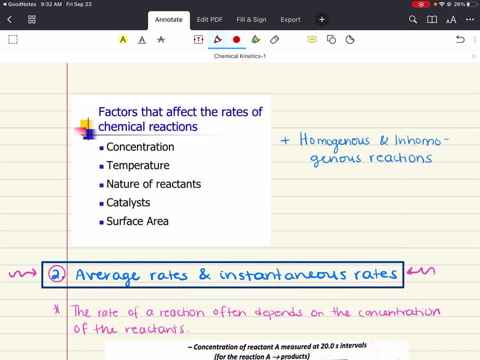 that influence chemical reactions. The higher the temperature, the faster the chemical reaction. Now, in addition to temperature, a second factor that can affect the rate of chemical reactions is the nature of the reactants. All right, Ions dissolved in aqueous solution, for example. 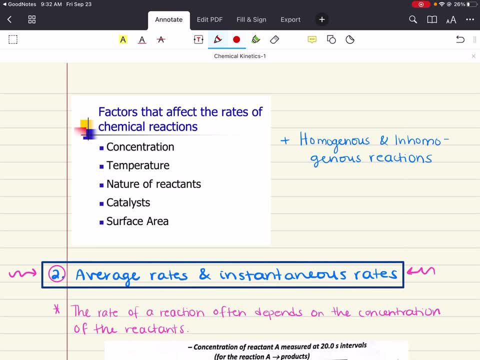 are going to react very quickly And that's going to affect the rate of chemical reactions, While covalently bonded molecules are going to react more slowly, All right. So the general rule is compounds with strong covalent bonds are going to react more slowly than compounds with weak. 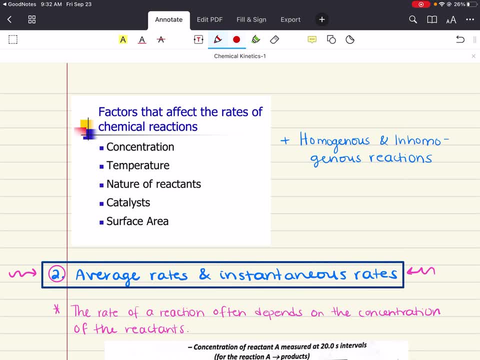 bonds And a larger molecule is going to often react more slowly than a smaller one. So that's another thing that can influence the rate of a reaction. Third, rate of a homogeneous reaction. Now, a homogeneous reaction is a reaction where all the substances are. 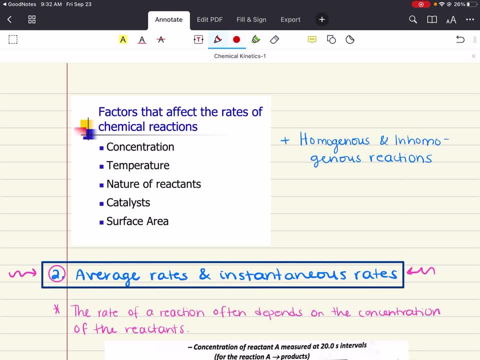 in this same phase, All right. And the rate of a homogeneous reaction is usually going to depend on reactant concentrations. A reaction can only occur when molecules collide. So in a liquid or gas, molecules can freely move around and they're going to collide with one another. 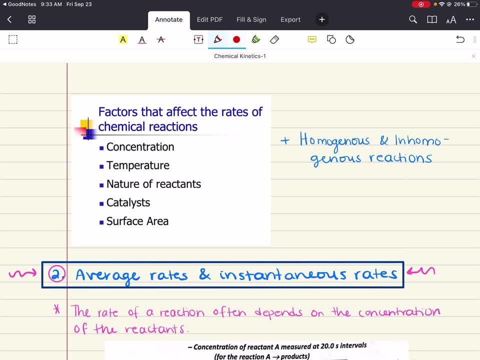 So at higher concentrations they're going to collide more frequently. That results in faster reaction rates. Now, what about heterogeneous reactions? Well, first of all, heterogeneous reaction is one in which the reactants are in different physical states- All right, And they can be really influenced by the state of subdivision. 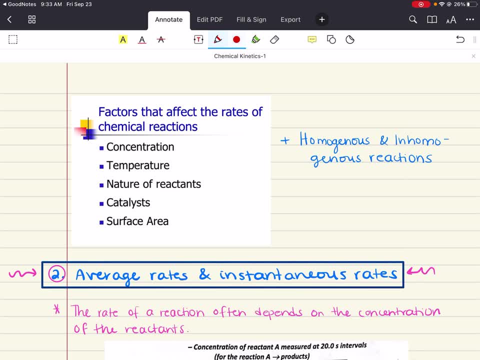 So what that means is reactions between a gas and a solid or between a liquid and solid. they're mostly going to occur at the surface of that solid, So the greater the surface area, the faster the reaction. All right, The last thing that we're going to cover. that actually. 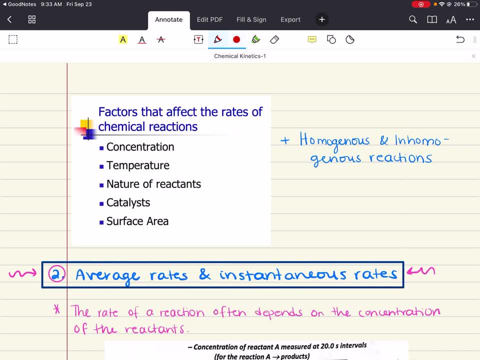 influences rates of chemical reaction are catalysts: the presence or absence of a catalyst. We're not going to say too much because we're going to cover catalysts in more details here in a few chapters. But a catalyst, in short, speeds up a reaction without being consumed. 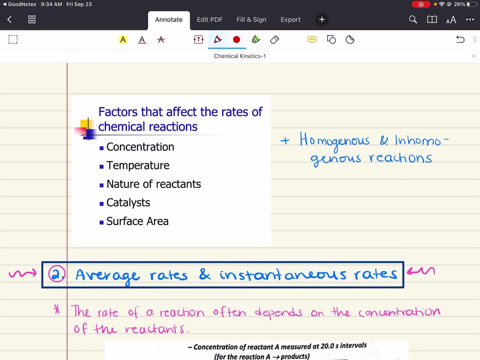 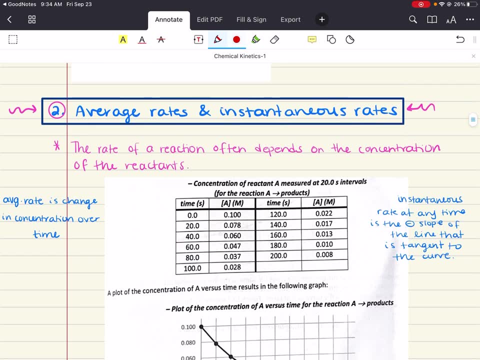 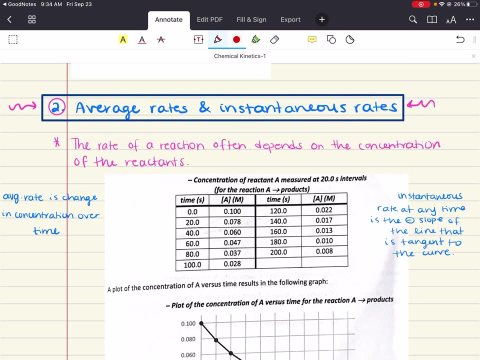 by the reaction. All right, So they're going to obviously, for that reason, influence the rate of chemical reaction. Fantastic. Now, with that being said, let's define average versus instantaneous rates. Reaction is going to depend on the concentration of the reactants, One way to analyze the relationship. 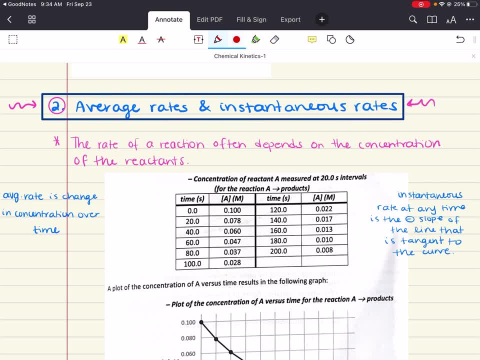 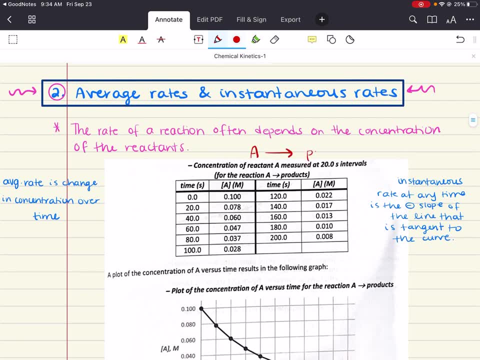 between concentration and rate is to plot the concentration of a reactant versus time. So, for example, what we have here is: pretend you have reactant A and it goes to product. What we want to do is measure the concentration of A at every 20 second interval. So we start initial time at. 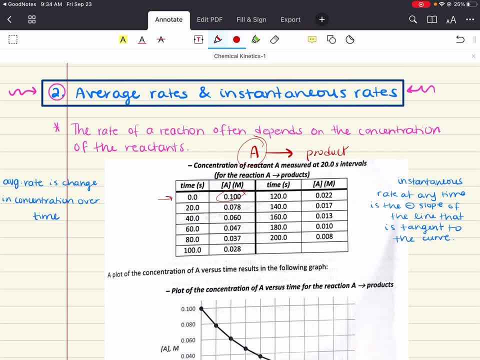 zero, We have 0.1 molar of concentration of A. Then after 20 seconds we start to measure the concentration of A. Then after 20 seconds we measure after 40, so forth all the way to 200. 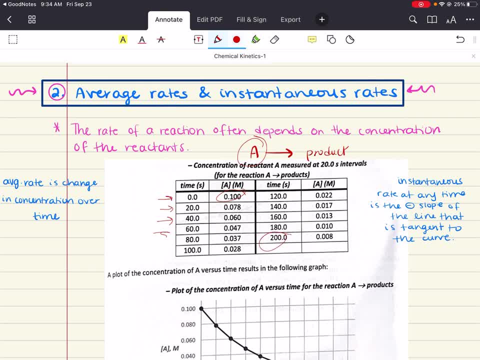 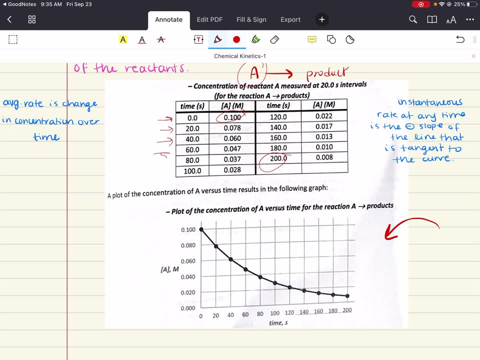 seconds. Then what we can do is we can plot concentration of A versus time and it results in the following graph here. All right Now, if we want to look at this graph and then kind of figure out the rate of the reaction. well, we know, rate of a reaction can be described for this reactant A. 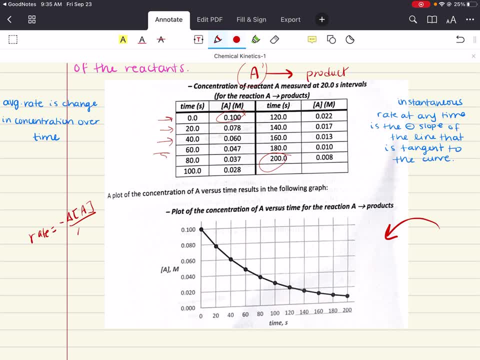 as minus change of reactant concentration of A over a period of time. All right, The average rate of a reaction over a certain time interval is going to be defined as the change in concentration divided by that time interval involved. So if we want to find the 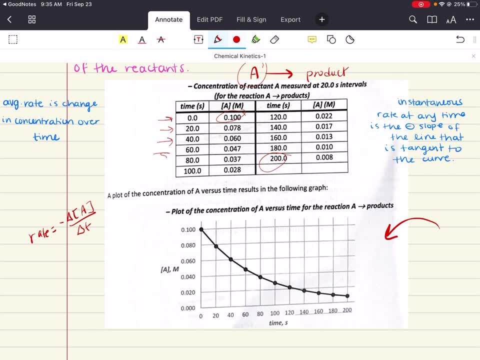 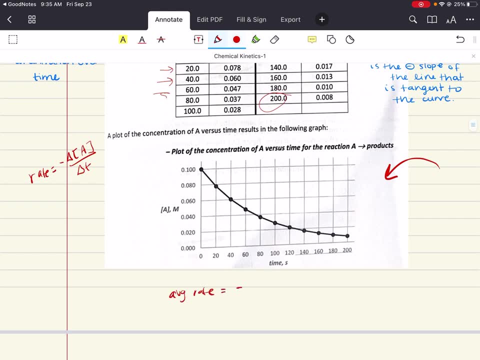 average rate of this reaction over the first 200 seconds. we can calculate that very easily by doing: oh, our average rate is going to be, well, the change in concentration of A over time. And if we're looking for the first 200 seconds, well, we're going to look at the. 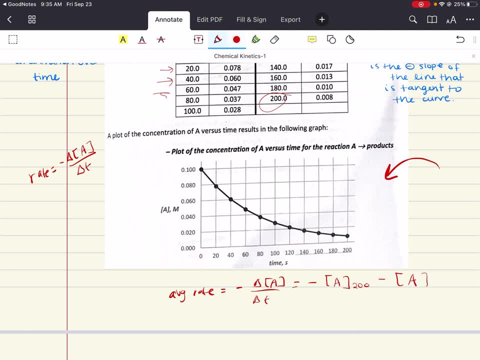 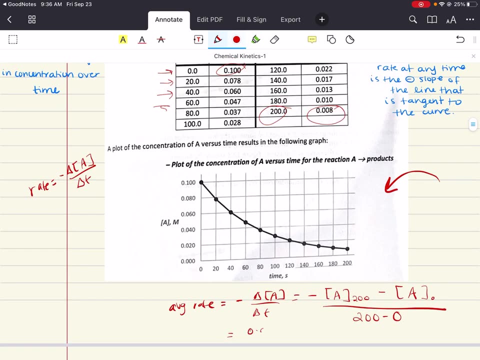 concentration at final minus initial, so at 200 and zero. and then we're going to subtract it by time. Our time is just 200 seconds minus initial seconds, which was zero. All right, What are the concentrations at 200 and at zero? At 200,, our concentration of A is 0.008, and our concentration 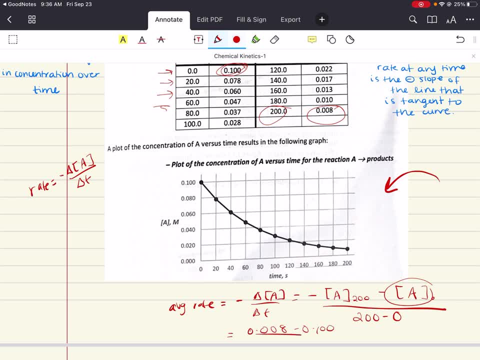 at zero seconds. initial is 0.1. Then we divide this by 200 seconds minus zero, Plug this into a calculator. You're going to get 4.6 times 10 to the power of 0.0. So we're going to get 0.0.. 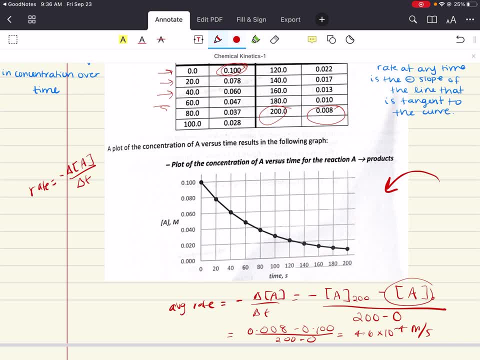 Minus 4 molar over second And we have figured out our average rate over 200 seconds for reactant concentration. A Fantastic. It's important to note now that the average rate is not the same as the instantaneous rate. The instantaneous rate is defined as the rate at a particular 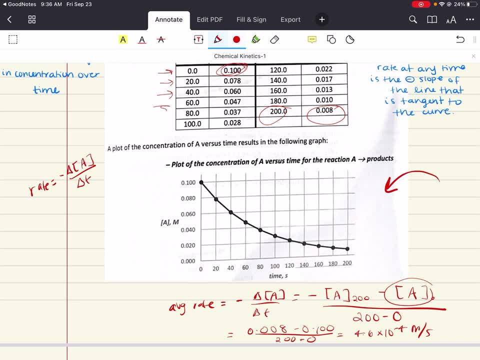 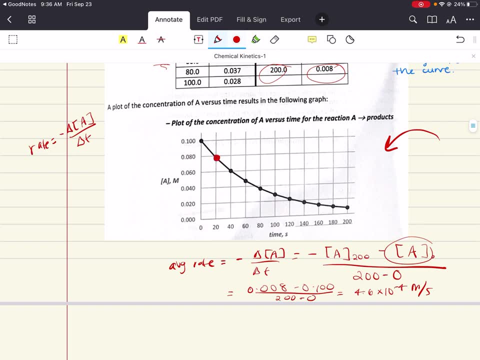 moment in time. How do we find the instantaneous rate? Well, the instantaneous rate at any point of time. So, for example, if we're interested in the instantaneous rate at 20 seconds, it is going to be the negative of the slope of the line that is tangent to the curve at that point. 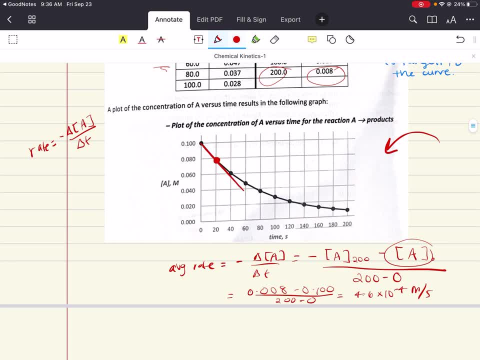 So we look at this point, We draw a negative slope line at that moment in time, All right, And the slope of that line tangent to that curve at that point, is going to be our instantaneous rate, All right. So to summarize, the average rate of a reaction, all right, is defined as the change. 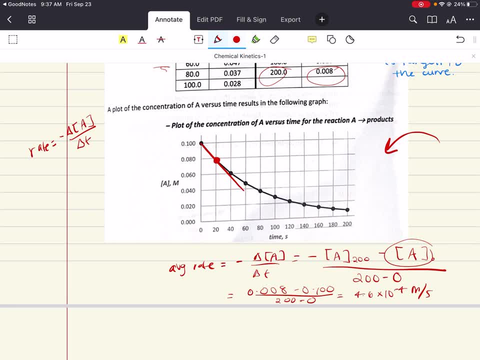 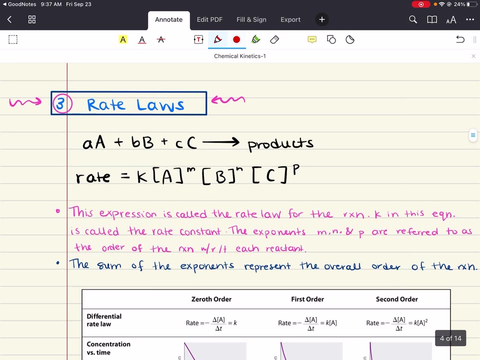 in concentration divided by the time interval involved. The instantaneous rate is defined as the absolute value of the slope of line that is tangent to the curve at that point in time. Fantastic. Now, with that defined, we want to jump into what the main topic of this chapter really is, And that is rate loss. All right For this reaction, all right. 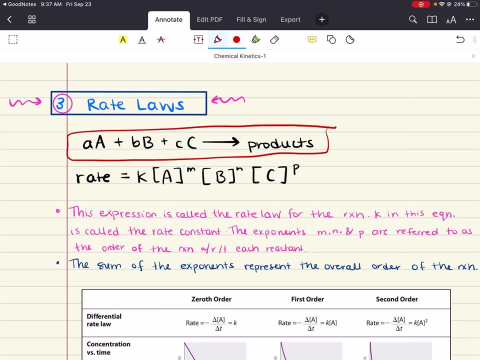 we're going to have this reaction as our starting point. All right, We have molecule A, B and C And there are coefficients- all right, to balance this equation- that are associated with molecules A, B and C. All right, For molecules A, B and C, we can say that the relationship between the reaction rate 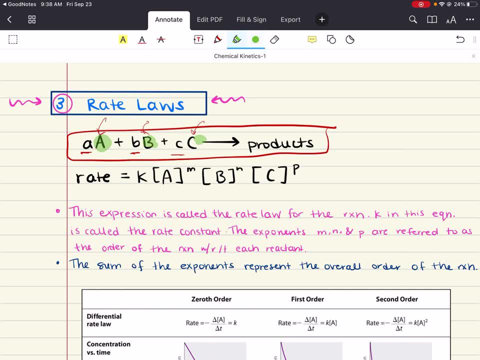 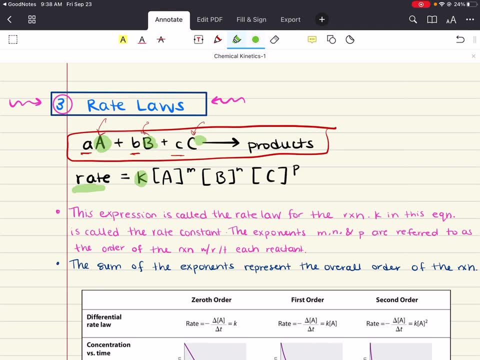 and the reactant concentrations can be expressed in the following way: The rate is equal to this constant- we'll say We're going to define it in a second- Multiplied by the concentration of A to some exponent. Multiplied by the concentration of reactant B to some exponent. Multiplied by the reaction. 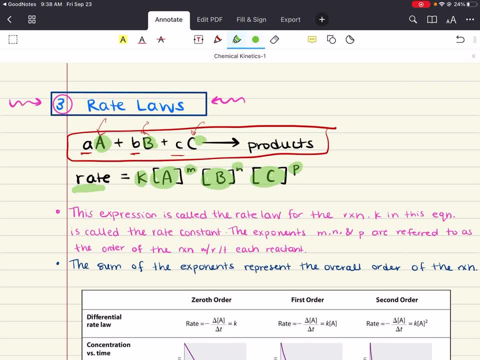 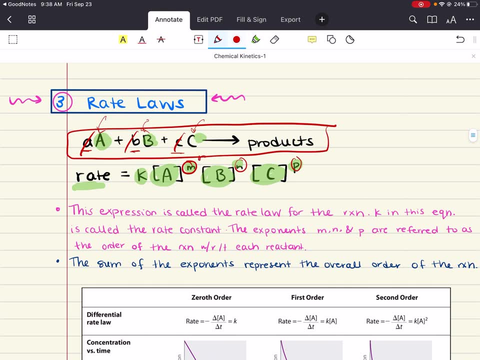 concentration of molecule C to some exponent. We do not know what these exponents are. They are not these coefficients, All right, But they are exponents associated with the concentrations of each reactant. This expression is called the rate law for this reaction. 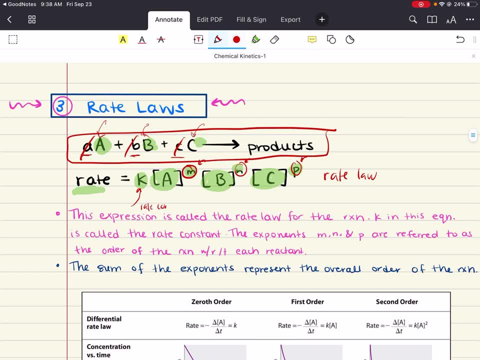 K is the rate constant. All right, It's a constant. A is the concentration of molecule A. It is raised to some. exponent These exponents: M, N, P. they are referred to as the order of the reaction with respect to each reactant. 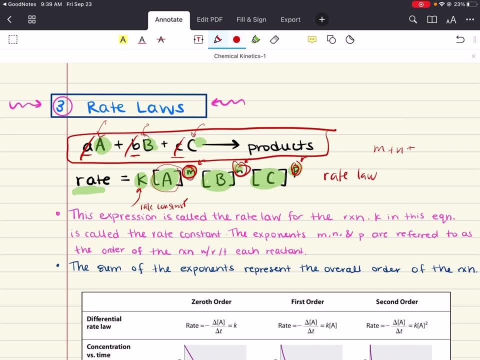 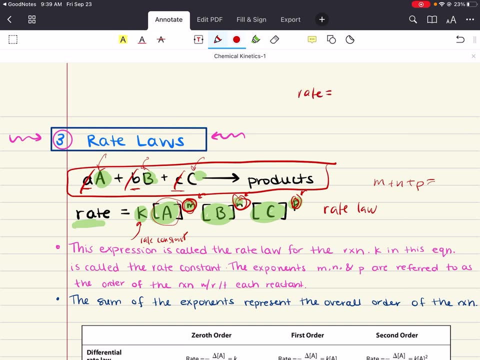 The sum of these exponents, if we were to add up M plus N plus P, is going to give us the overall order of the reaction. So let's do a few examples. Let's say, for example, we're trying to write the rate law for a reaction. that is first order in A, first order in B. 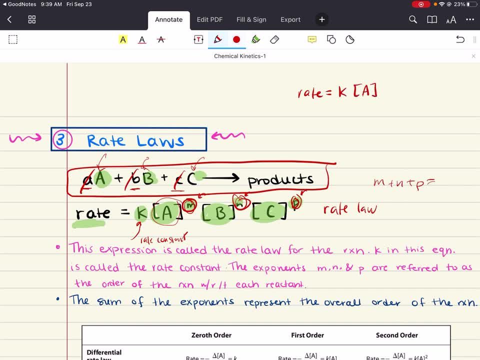 We write our rate constant. Then we write the concentration of reactant A. They told us it was first order, So we associate an exponent one with this. And they told us that the reactant B is also order one, So we associate a one exponent with that. 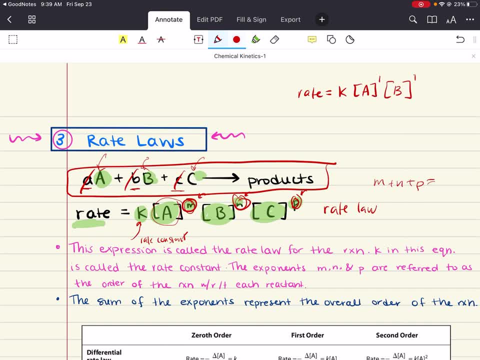 What is the overall order of this reaction? It is simply going to be the addition of both those exponents, So one plus one is two. The overall order of this reaction is two. Fantastic. Now let's look at a reaction that has only reactant A, and reactant A is second order. 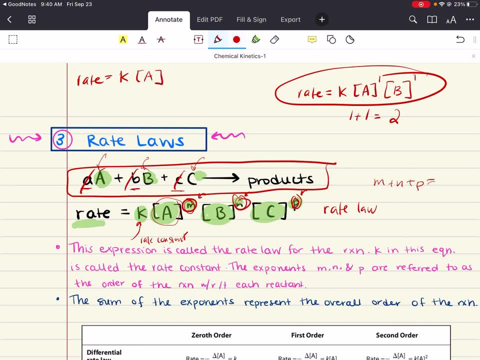 Let's write the rate law K, concentration of A, and it is second order. Fantastic, That is the only reactant we have and it is second order. So the rate order of the whole, the overall order for this reaction, is also still just two because there's no other reactant. 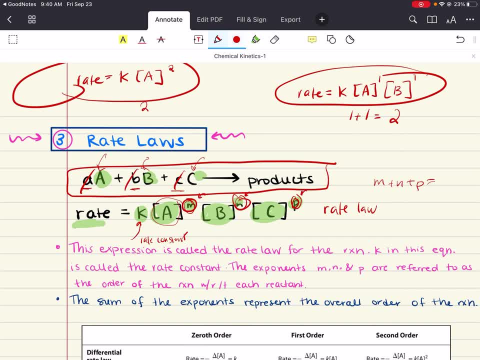 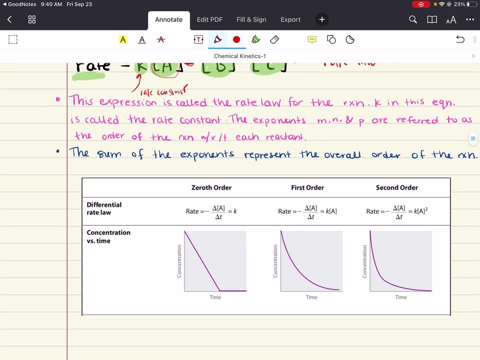 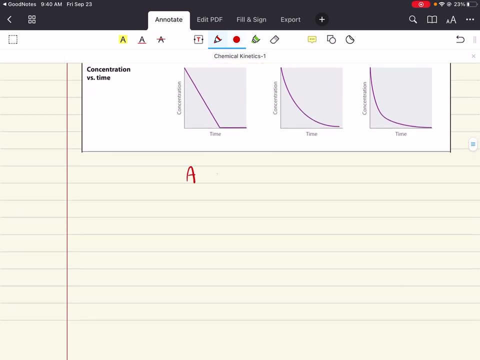 with any other exponents. Now, there are many different rate laws, And three of the reaction types that we're going to frequently encounter are first order, second order and zero order reactions. To talk about these, what's going to motivate our conversation is well, we're going. 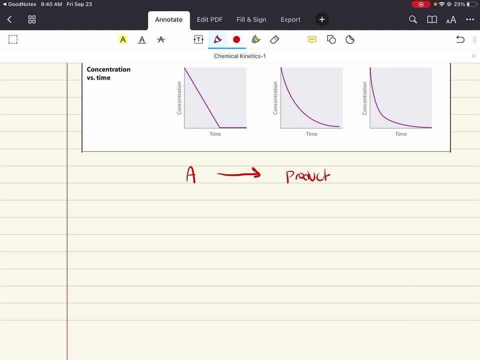 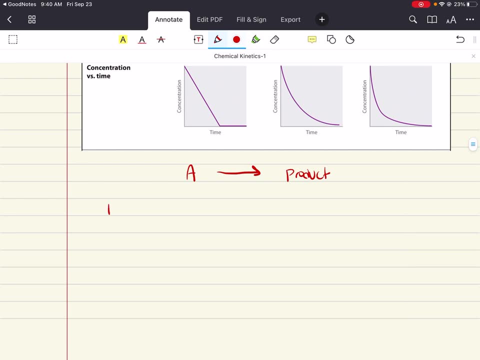 to have reactant A. that goes to products. All right, It is first order that this reaction is first order with respect to A. All right, So let's pretend this is a first order. Let's write the rate law. The rate law is going to be equal to. 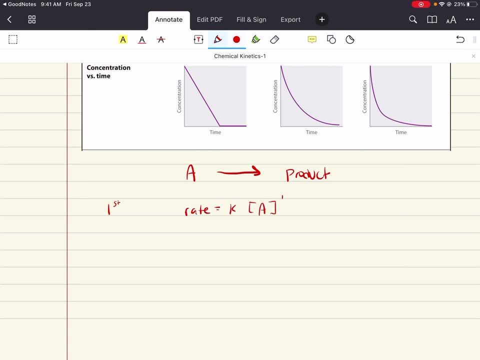 the rate, constant times the concentration of A and it is first order, So we're going to give A the exponent one In first order reactions. the rate of the reaction is directly proportional to the concentration of reactant. What does that mean? 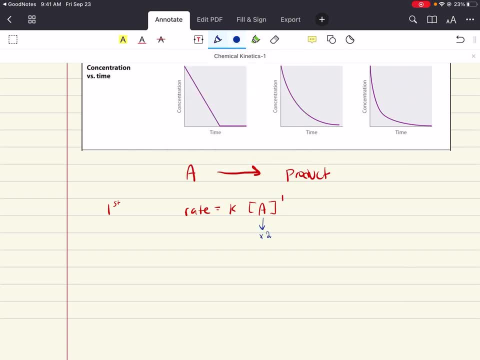 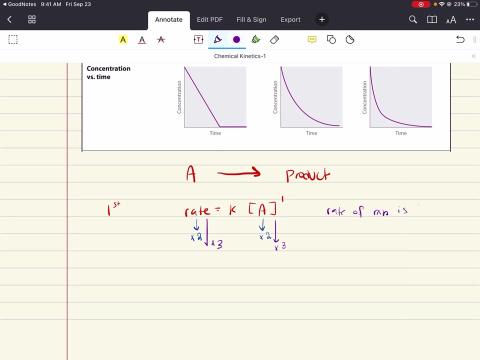 That means if we double the concentration, the rate is also going to double. If we triple the concentration, the rate is also going to triple. So the rate of reaction for first order is directly proportional- I'm going to write proportional, like that- to the concentration. 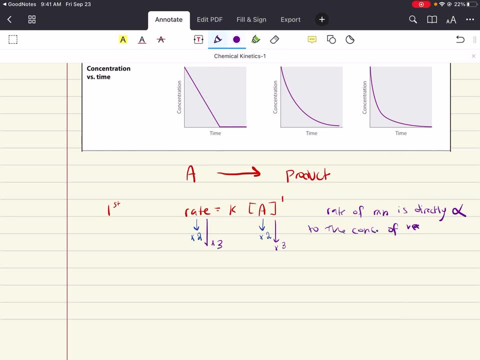 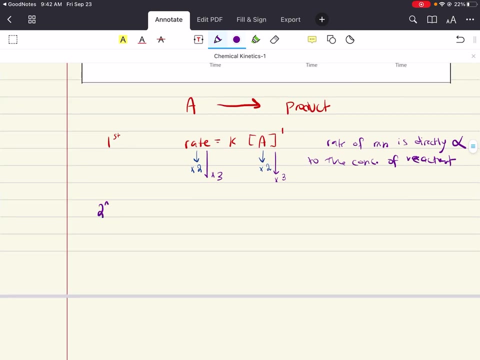 of reactant. All right. So if you double A the concentration, you double the rate. Triple the concentration. triple the rate. Quadruple the rate, the concentration, quadruple the rate. Fantastic. Now what about second order? Let's write this reaction's rate law, if it was second. 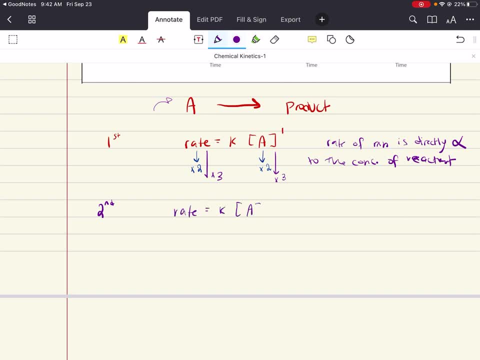 order We're going to write. rate is equal to K, concentration of A to the second exponent. All right, This is the rate law. In second order reactions the rate is directly proportional to the square of the concentration. So if we multiply the concentration by two, the rate is going to increase to the square of two. 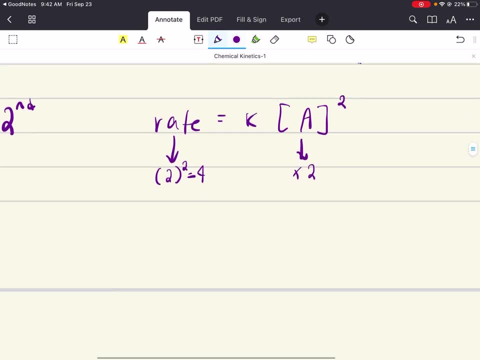 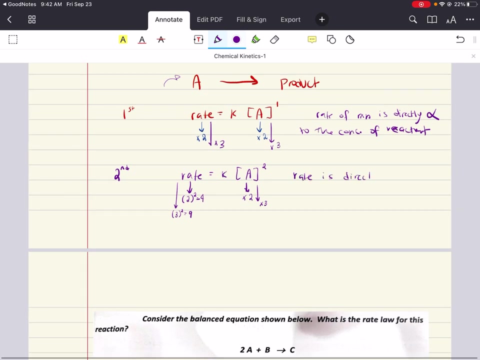 So it will quadruple? All right, If we multiply the concentration by three, the rate is going to increase by three squared, So nine times over. All right, So the rate is directly proportional to the square of the concentration of reactants. All right, Fantastic. What about? 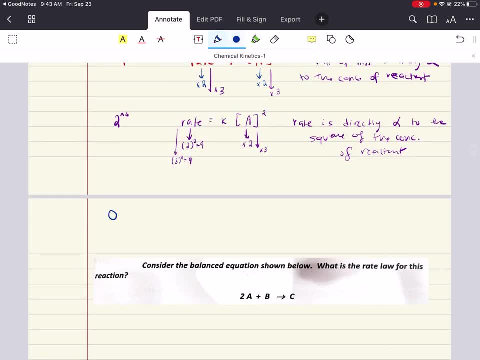 zero order. All right, Zero order. Let's write the rate for zero order, K, concentration of A with a zero exponent. Now, anything to the exponent zero is just one, And so the rate is really only dependent on the rate constant and not the rate constant. So if you double A, the rate is going to. 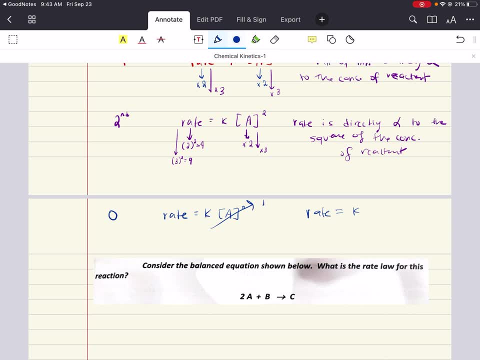 be dependent and not the concentration. So for zero order rate laws. any change in the concentration of A does not affect the rate at all. So change in concentration of A or reactant- Sorry, my handwriting is bad- Will not change rate law. All right, Because it's not dependent on concentration. 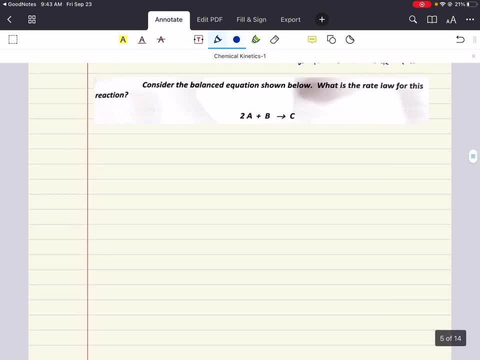 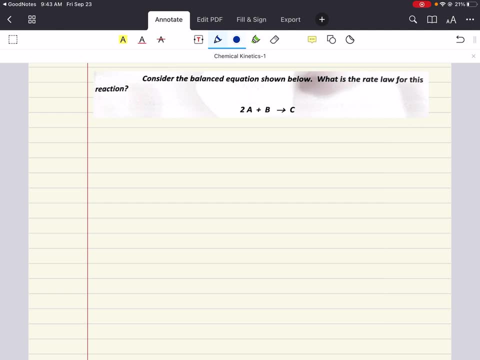 whatsoever. All right, Fantastic, Let's put this into action here. All right, Let's put this into action. Consider the balanced equation shown below: What is the rate law for this reaction? This is what we say, a trick question, because the answer to this problem is technically there's not enough. 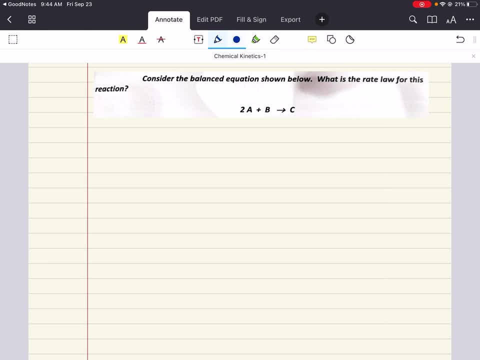 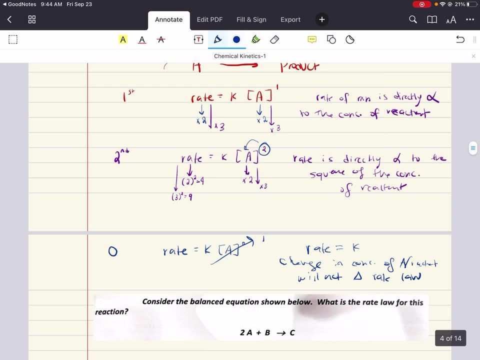 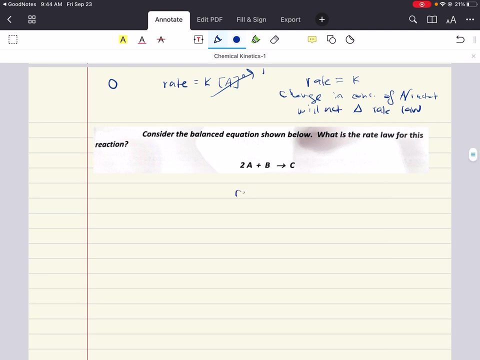 information to determine the rate law for this reaction, Those exponents that are associated with reactants, all right in. rate laws are not determined from a balanced equation. They are determined experimentally. You cannot write the rate law for this equation as K equals. 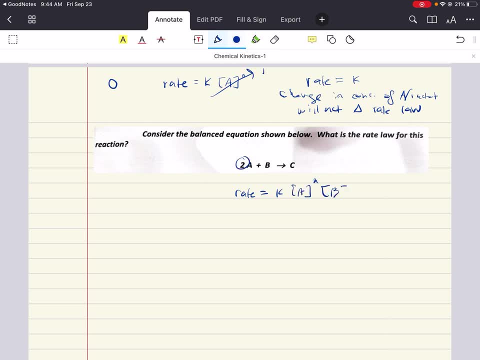 concentration of A to 2, concentration of B to 1.. That is incorrect. That's not how you figure out the rate law. That's not how you figure out the exponents associated with the reactants concentrations. You have to experimentally figure that out. So this would be incorrect. You cannot. 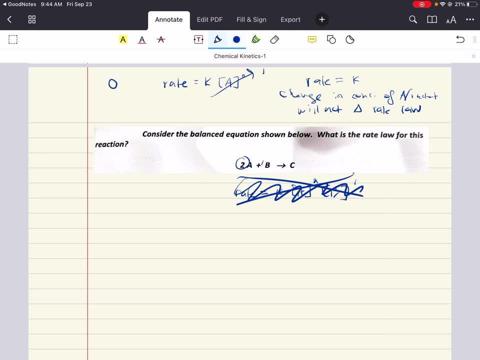 write it like that, All right, And so technically, the correct way to answer this question is to say there is not enough information. The only thing we can write is that the rate law is equal to K. concentration of A to some exponent we don't know. concentration of B to some exponent we don't know. 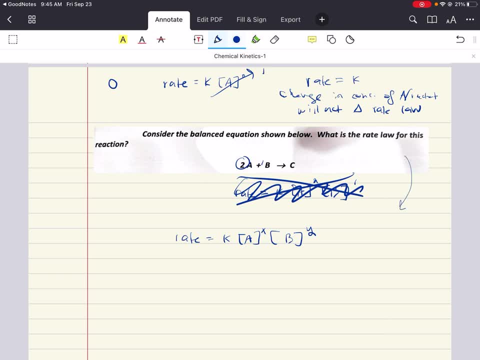 All right. So this is a kind of trick question that your professor might ask as a multiple choice question to throw you off. Make sure you know you cannot tell. you cannot write a true rate law just based off of a balanced equation. That is not enough information. 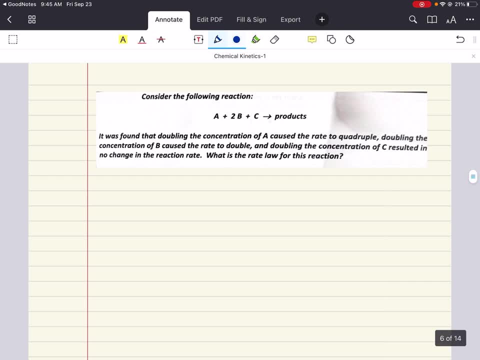 Fantastic. Let's do one more practice problem here. All right. This problem says: consider the following reaction: All right. It was found that doubling the concentration of A caused the rate to quadruple, doubling the concentration of B caused the rate to double and doubling the 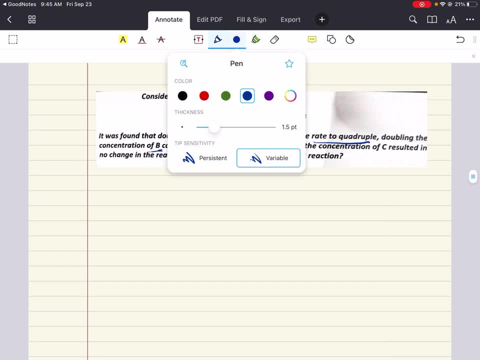 concentration of C resulted in no change at all. All right, So let's write the structure of this rate law and then go through this one by one. We have K rate constant times reactant concentration A times reactant concentration B times reactant concentration C. 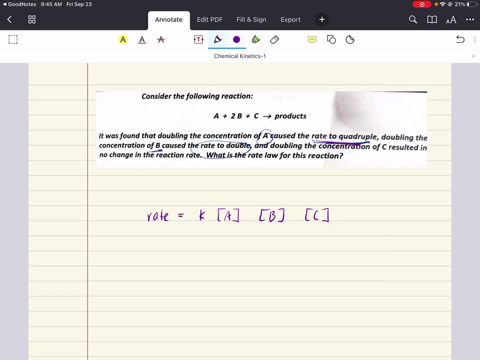 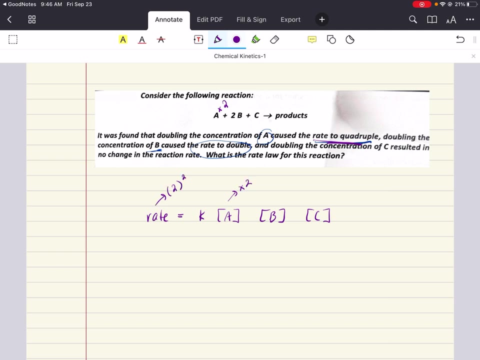 now, based off of this information, we can hopefully determine the exponents associated with both. let's start with a. when we doubled the concentration of a, all right, the rate. the rate changed by two squared, so the, so the, the, the square of the concentration. we know what that describes. 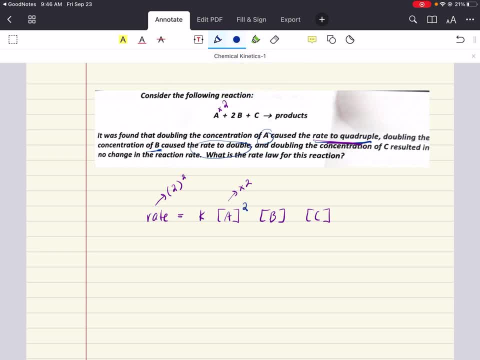 that describes a second order. all right, and so a is um. the order of reaction for and with respect to a is second order. what about b? doubling the concentration of b resulted in the rate to double. all right, we know that this describes a first order reaction, so the exponent associated with 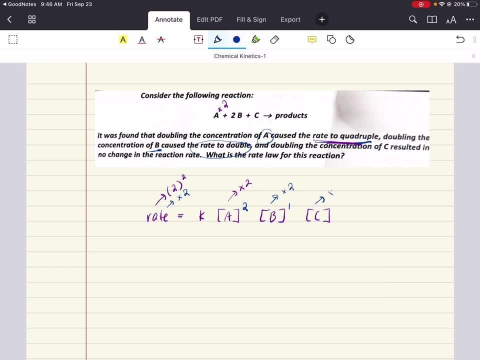 b is going to be one. what about c? we doubled c. nothing happened to the rate. this is a description of a zero order reaction. all right, so there we have it. we've written the rate law for this reaction. the question, though, asks: what is the rate law for this reaction? and also, i want to add, what? 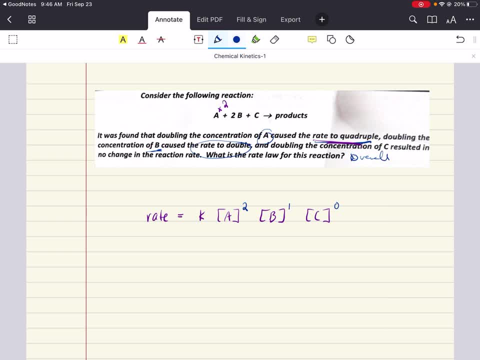 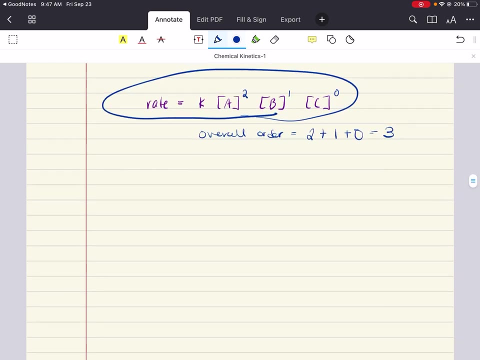 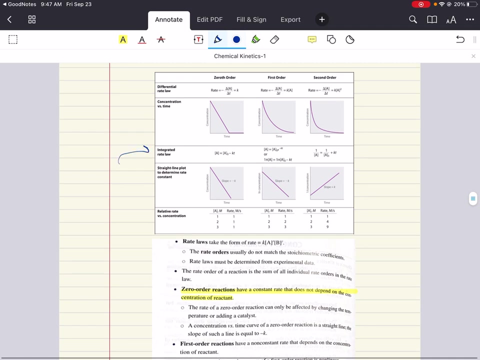 is the overall order of this reaction. to figure out the overall order, we just have to add the exponents two plus one plus zero. that's three. this reaction is overall. third order: fantastic you all. right now this is kind of a summary page and we're gonna get into some of the details of this. 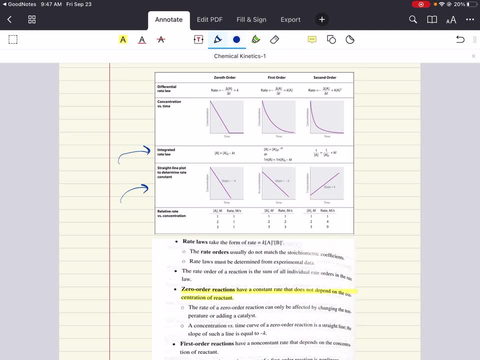 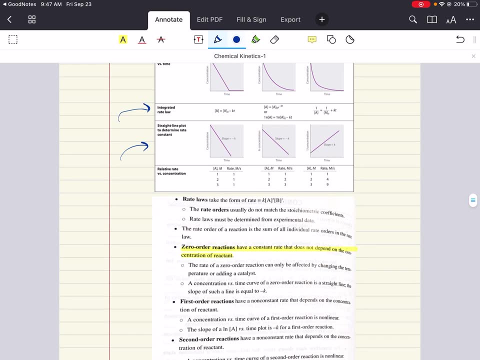 figure here, um, as the second topic and the second topic in this uh chapter that follows rate laws is integrated rate laws. all right, but first i want to also talk about how we can obtain the rate law first, before we talk about integrated rate law. just from initial rate data, i told you. 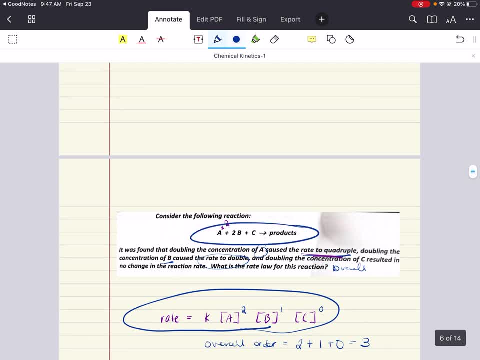 you cannot look at the rate law first and then you cannot look at the rate law first and then you cannot look at a, a balanced equation, and write a overall rate order. all right, that is not enough information because you cannot use these, these, these coefficients, as exponents. but if you collect, 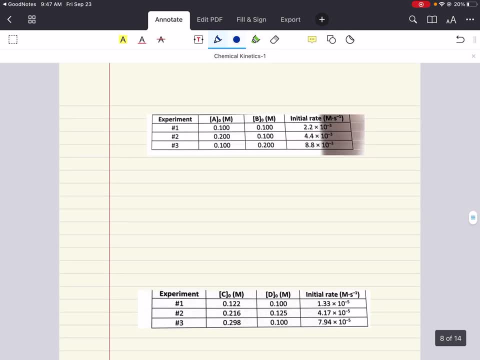 rate data. all right, if you collect rate data, you can then obtain the rate law from that. so what we're going to do is do exactly that. all right, let's look at this first box right here. one way to determine the rate law first is to look at the rate law first, and then you can look at the rate. 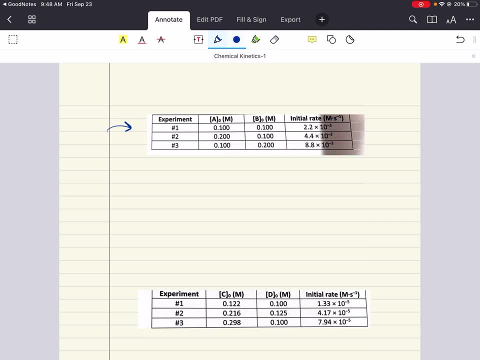 law for a particular reaction is to measure the initial rate while you vary the initial concentrations of the reactants. so what we have is a reaction. a plus b is going to equal product. so we have two reactants here. in our first experiment we kept both at the same concentration and we 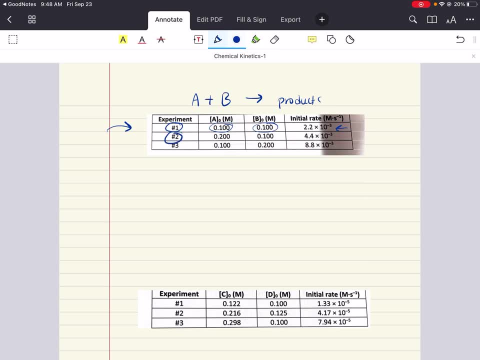 figured out their initial rate. in our second experiment we kept the, the concentration of b the same, but we doubled the concentration of a. so here we doubled the concentration of a. so here we doubled the concentration of a only, and then we observed the initial rate. now we can compare the. 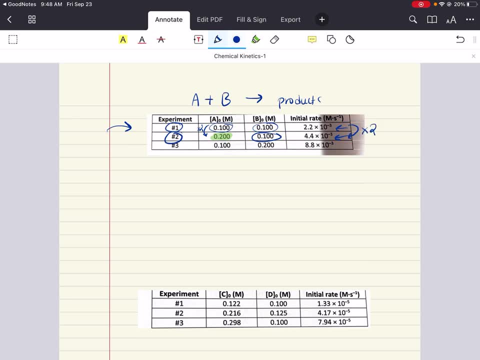 rate of one and two and see how it changed. well, it doubled. when we doubled the concentration of a, we also doubled the rate. so what did we just figure out? that a is first order, all right, fantastic. now what if we look at experiment three? in experiment three, we keep the concentration of 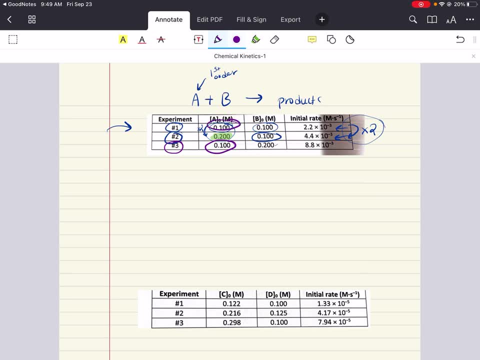 a, the same as we did in experiment one, but then we doubled the concentration of b from the first experiment. so we multiply by two, then we measure the rate for experiment three and we can now compare it to experiment one and we can note the difference: it has quadrupled. so when we doubled the, the concentration of b, the rate. 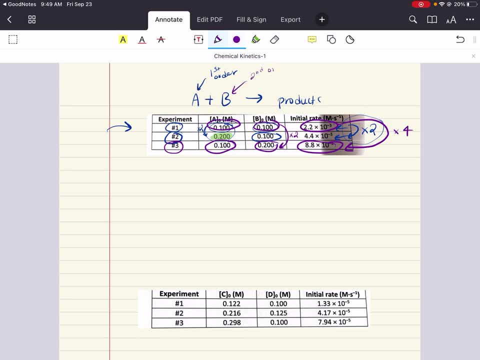 quadrupled, that means b is second order, and that means when we rate the write, the rate law for this, we write k, a to the first order, b to the second order, and that's it. now, what i'm going to do is i'm going to let you figure this. 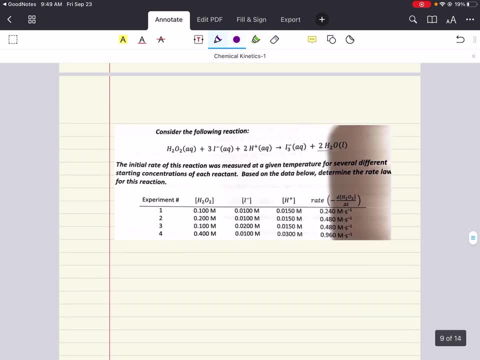 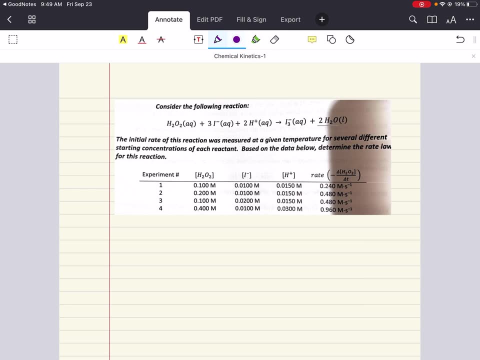 out. but what's going to help you figure this out is an example problem we're actually going to do together. all right, this example problem says: hey, look at this reaction. what we're trying to figure out for this reaction is the following: the initial rate of this reaction was measured at a given 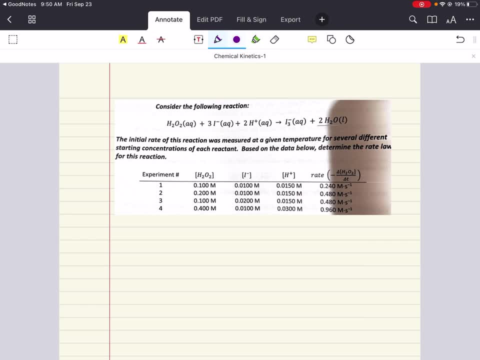 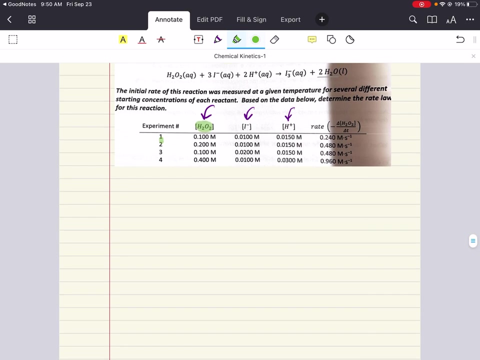 temperature for several different starting concentrations of each reactant, based on the data below, determine the rate of this reaction. perfect. we have three reactants- hydrogen peroxide, iodine minus and h plus, and we have conducted four experiments. let's start by figuring this hydrogen peroxide rate first of all. all right, experiment one. we have these following: 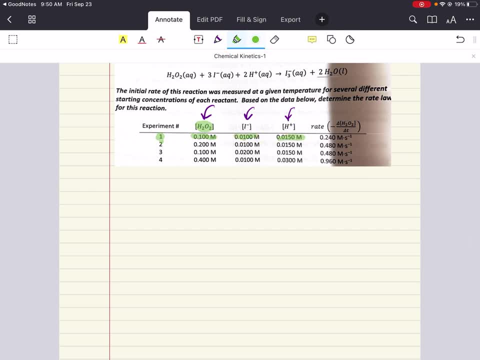 concentrations. cool beans. let's try to find an experiment to compare it to that keeps the concentration of iodine and h plus the same, and we're going to compare it to the concentration of hydrogen peroxide. which one of these would do that experiment? two: all right, the concentrations. 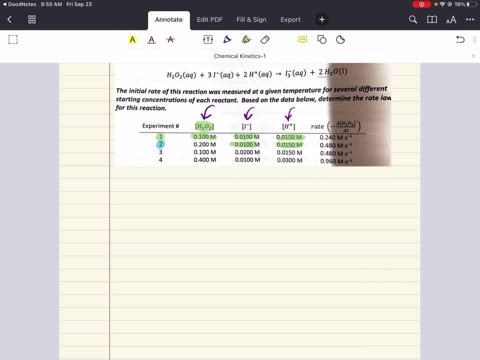 of iodine and h plus are kept the same. the only thing that changes is the concentration of hydrogen peroxide. this is going to allow us to do a direct comparison here. we multiply the concentration of hydrogen peroxide by two, and then what happens to the rate as a consequence? 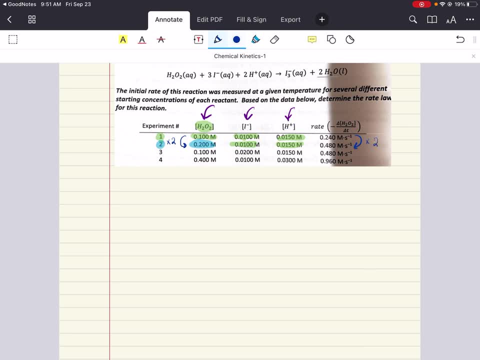 it also gets multiplied by two. so we're going to do a direct comparison here. we multiply the by two. what does that mean? that means hydrogen peroxide is first order- fantastic, so we figured that one up. let's move on to iodine. all right, let's move on to iodine. let's erase this, all right. 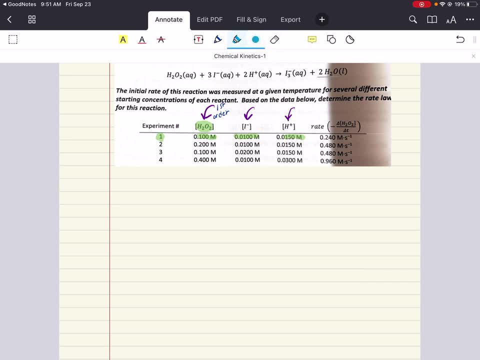 let's look at that first experiment. let's find another experiment that keeps the concentration of hydrogen peroxide and h plus the same, all right, but changes the concentration of just iodine. that would be experiment three. let's compare experiment one and three. all right, here we have doubled the concentration of iodine. 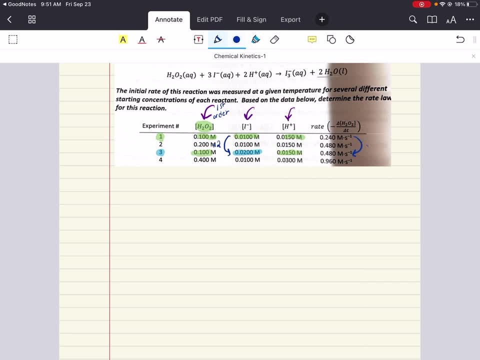 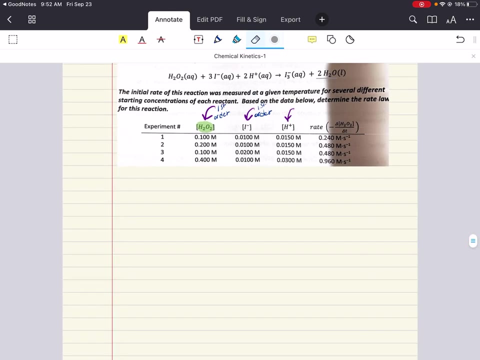 what happens to the rate? it also doubles. what does that mean? that means that iodine is also first order. fantastic. now we want to figure out the order of h plus. this is the only thing that we have left. the problem here is that we don't have any. the only experiment where we change the 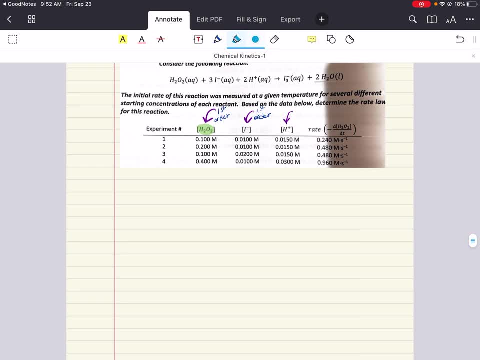 concentration of h plus is experiment four. that's the only experiment where h plus concentration is changed. look at one through three. nothing changes in the concentration. so that means we have to use experiment four. cool, because that's the only one where the change in concentration for h plus. 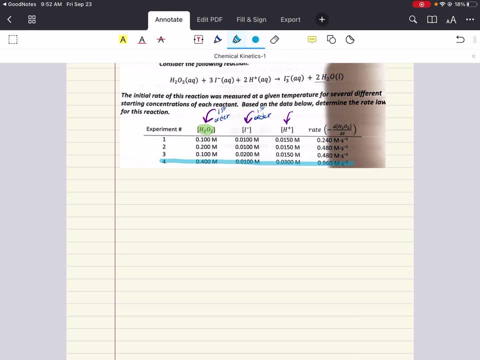 happens. but then we can't find another experiment where we keep everything else constant. everything else also changes, and so we're going to have to use a different technique. let's just choose another experiment to compare it to. i'm just going to choose two you can choose. 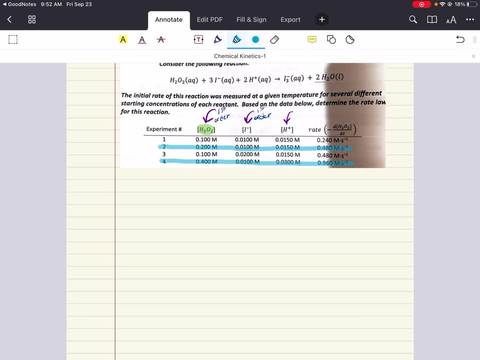 any really, and you're going to get the same answer. i'm going to compare experiment two to experiment four. all right, what is happening between these two experiments? well, the concentration of h plus is doubled, but also the concentration of hydrogen peroxide is doubled. that means we 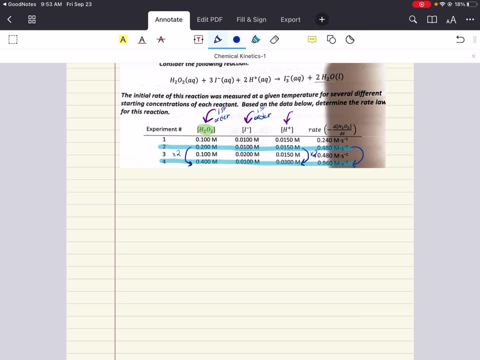 cannot just look at the rate and conclude: what is the order of h plus? what we have to base this off is off of a ratio. all right, what we're going to do is we're going to set up a ratio of the rate data for experiment two and four. so what that means is we're going to write the rate law. 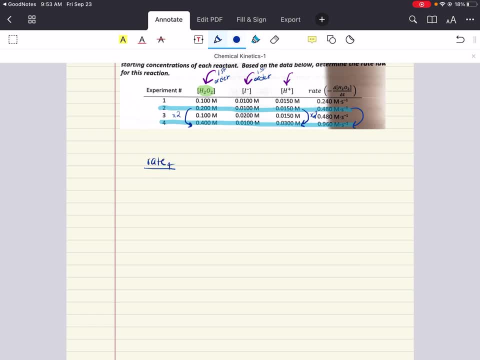 for experiment four. and then we're going to write the rate law of experiment two over that- i mean under that. so it's rate law of experiment four over the rate law of experiment two. so let's do just that. what is the rate law for experiment four? it's the rate. 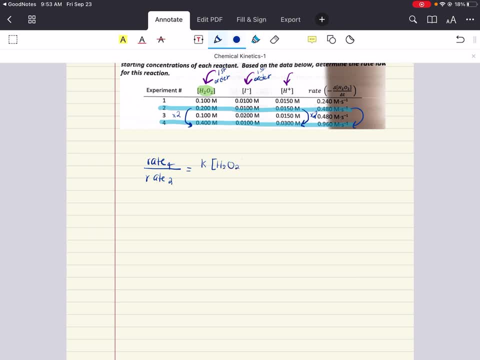 constant. all right, we have hydrogen peroxide. we know it's first order, so we're going to give it the first order. all right times iodine: all right, which is also, which is also first order times h plus we don't know what. the rate order of this is cool, then we're going to rate right over this. 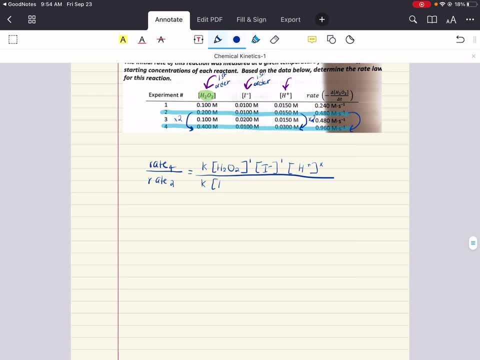 the rate law for experiment two. it's going to be the rate constant times: hydrogen peroxide to the first order, iodine also to the first order and then h plus. we don't know the order of that yet. that is okay. what we're going to do now is fill in the blanks. 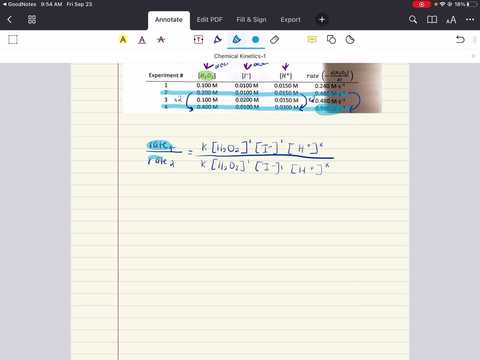 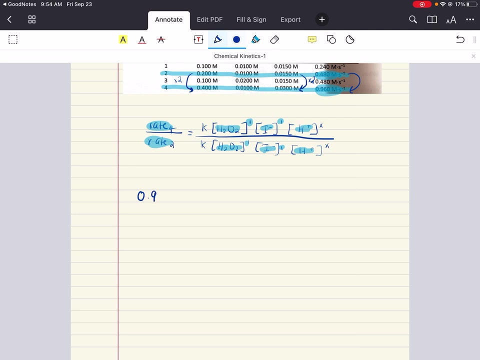 for everything. we know. we know what the rate of experiment four is. we know what the rate for experiment two is. we know the concentrations of everything and the orders for two of the reactants out of three. let's plug things in. what is the rate of experiment four? it's 9.960 over the rate. 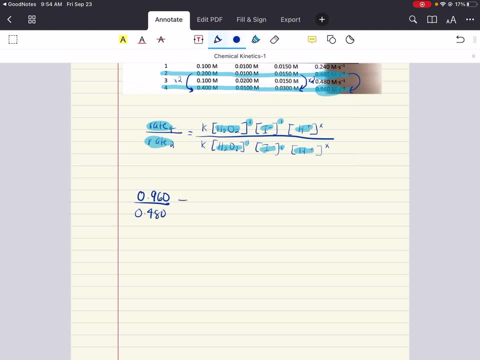 of experiment. two: zero point four, eight zero, all right. rate constants, all right. what's the concentration of h202? and four, it is 0.4. to the power of one iodine is 0.01. to the power of one h plus is 0.03. we don't know what the rate order is. 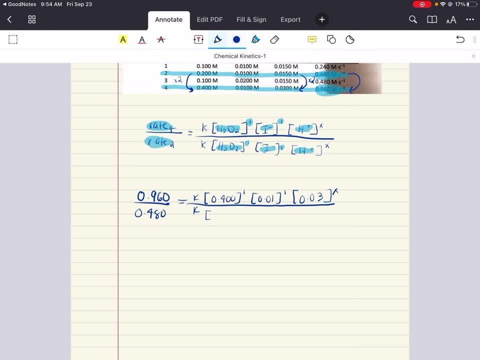 here. now for experiment two. what is the concentration of hydrogen peroxide? 0.200 to the power of one, iodine is 0.01 to the power of one and h plus is 0.015. we don't know what the order is. notice things. cancel out really quickly. these. cancel out, these. cancel out. this simplifies to two. 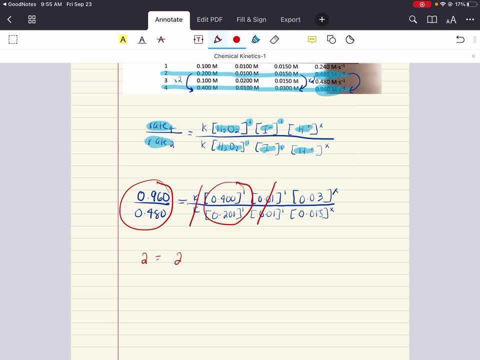 this also simplifies to two, and then what we have here is just 0.03 over 0.015 to the x exponent. this also simplifies, and it simplifies down to two. all right, what we're going to do here is then we're going to write: two is equal. 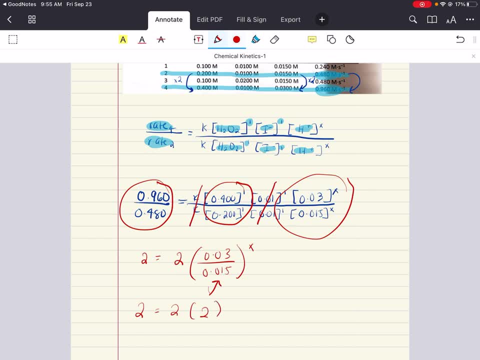 to two times two to the x power. now we're going to divide both sides by two, so these cancel out, and what we have here is one is equal to two to the x power. how are we going to make this true? the only way to make this true is if x equals zero, because anything to the power. 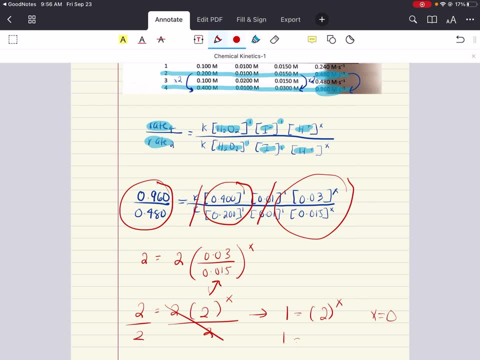 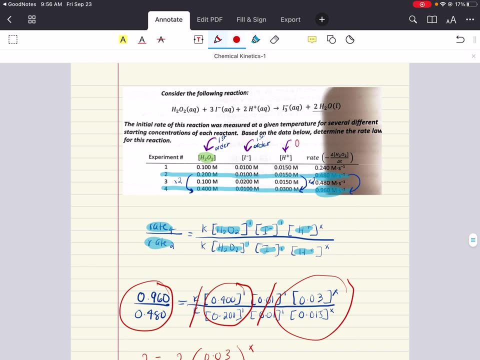 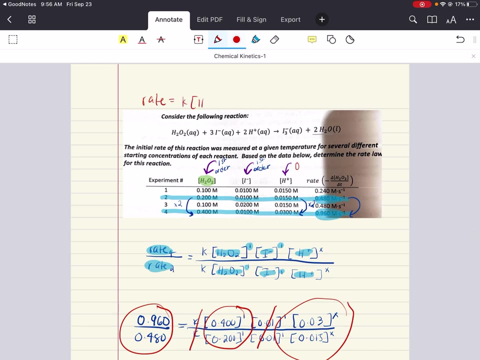 x is just one, and so then you get one equals one, and that is correct. what does that mean? that means the order of h plus is zero order. and now, if we write the rate law for the entire reaction, the rate law is just going to equal x- hydrogen peroxide- to the first order, iodine minus to the first order and h plus to the.